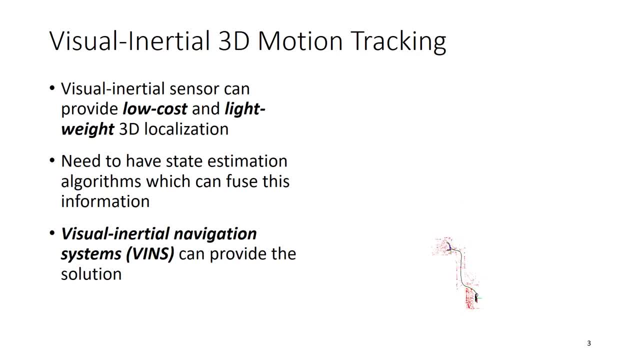 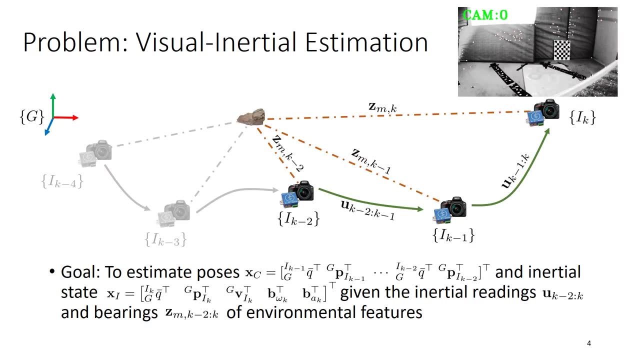 Visual inertial sensors can provide a very low cost and lightweight 3D localization solution. We need to develop state estimation algorithms which can efficiently fuse this information together, and this class of algorithms is generally termed visual inertial navigation systems. So the key problem that we're trying to solve in visual inertial estimation is we're trying to estimate a historical series of poses through the environment of the camera IMU system. 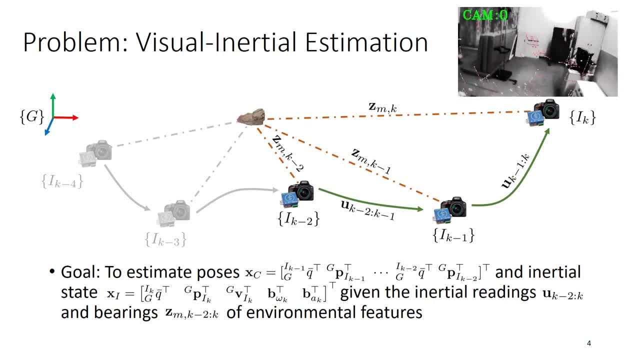 So as the camera and IMU move from one time step to the next, so, for example, from IK minus two to IK minus one to IK, it collects both inertial measurements, in this figure denoted as U, from one time step to the next. 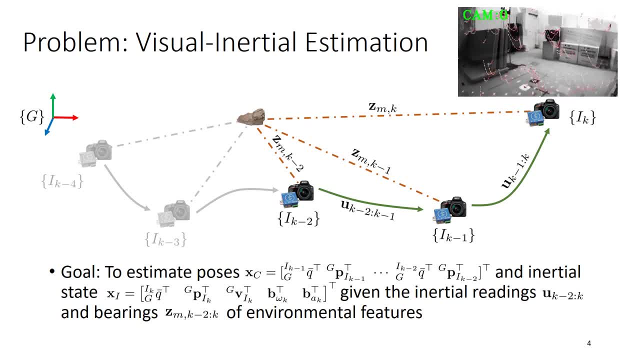 And, additionally, it collects visual bearing information to environmental features, in this case denoted as ZM, And the goal is to estimate the historical poses, the orientation and position at each one of these time steps, along with an initial state given these inertial readings and bearings of the environmental features. 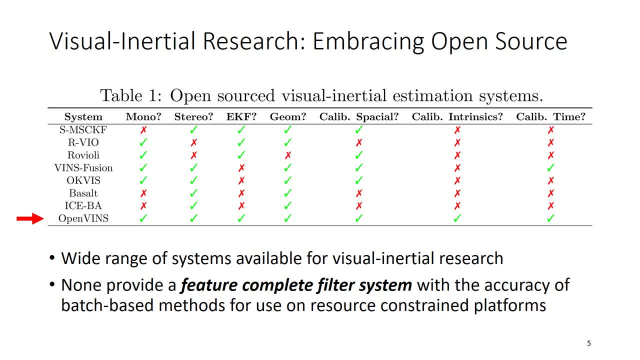 So, while we looked at the existing visual inertial open source landscape, there's a wide range of great systems available to perform visual inertial research on top of, But none of these provided a feature complete filter system with the accuracy of the batch based methods for use on resource constrained platforms. 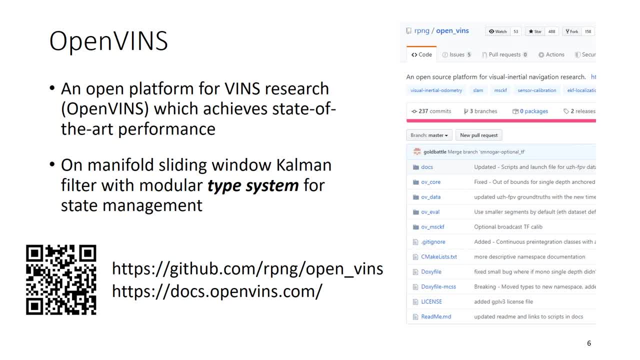 And so this is where the OpenVINZ project comes in. OpenVINZ is an open platform for visual inertial research which achieves state-of-the-art performance, And under the hood it's an on-manifold sliding window common filter with a modular type system for monitoring visual inertial research. So all of this is going to be implemented on an open platform like MonsterVide, And so we got that set up for evaluation. We got that set up for evaluation. So all of this is going to be implemented on an open platform like MonsterVide. 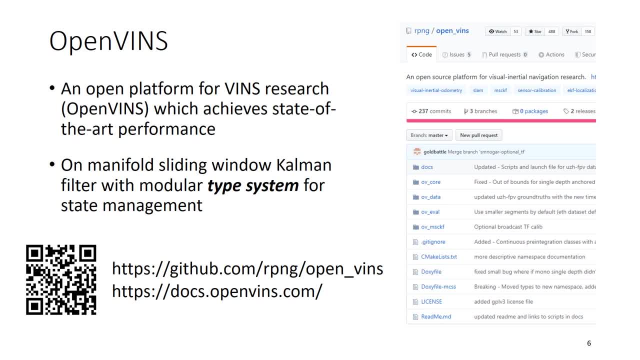 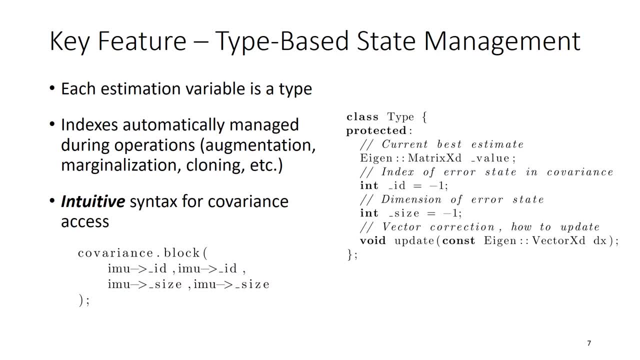 for state management. please check out our github here and and our documentation website. so one of the key features to our system is a type based state management. each estimation variable that we're trying to estimate is a type and the index into the location of the covariance automatically managed during covariance reordering operations, such as 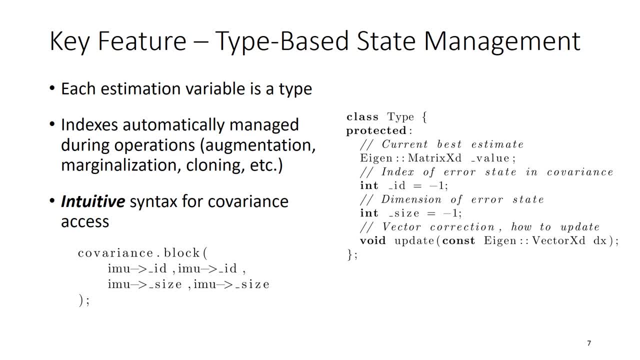 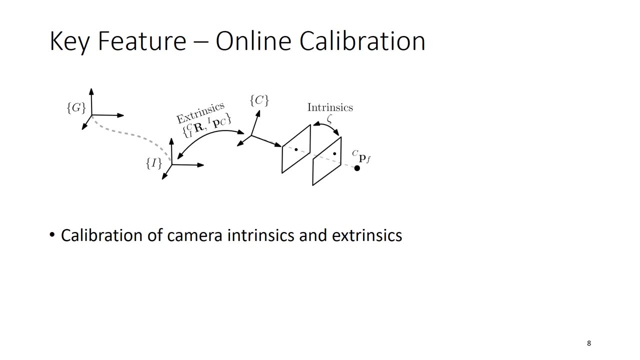 augmentation, marginalization, cloning. what this index c or id management does is it allows for intuitive syntax into the covariance. another key feature is the ability to perform online calibration, so we have a very complete measurement model and so we can calibrate the camera intrinsics and extrinsics. and another important thing that we calibrate is we calibrate the temporal offset. 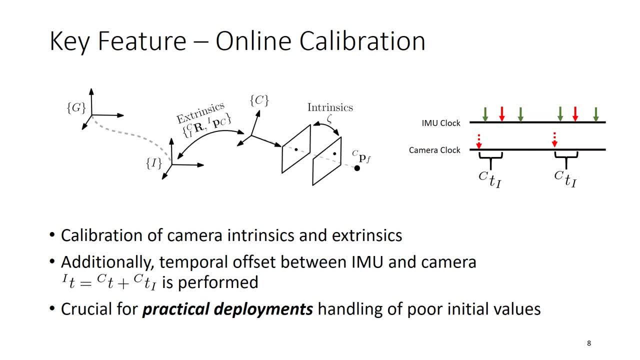 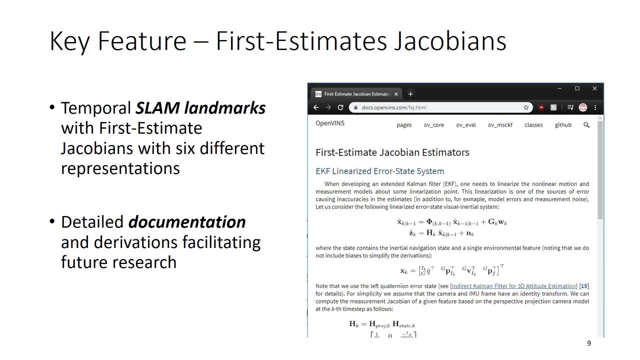 between the imu and camera, and both these are very crucial for practical deployments and handling of very complex and complex operations. and so we can calibrate the camera, intrinsics and extrinsics- very poor initial calibration. Another key feature is the use of temporal slam landmarks and ensuring proper consistency with first estimate Jacobians. We have six different. 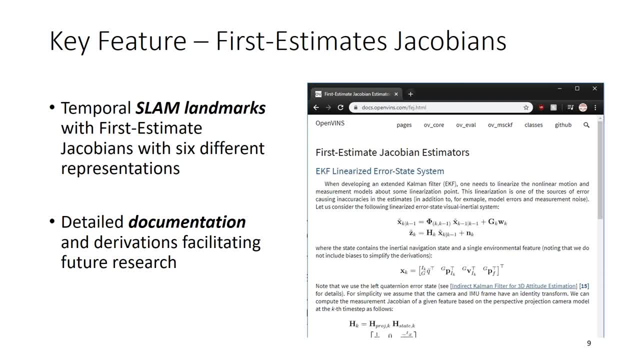 representations with different trade-offs in accuracy and efficiency. Along with this, another important part of the project is very detailed documentation and derivations, And so there's a whole documentation website where we have our derivations and how we get specific equations And the idea there is, so anybody that's coming to the code base can look. 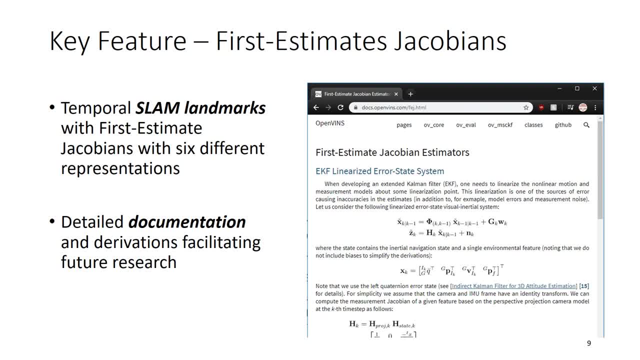 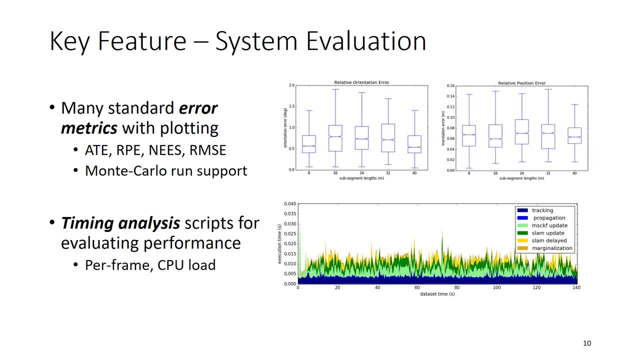 at the documentation website and instantly become familiar and understand what we're doing in the code. Another key feature is our system evaluation toolbox. We include many different standard error metrics, including AT, RP, RPE, et cetera. We additionally include timing analysis scripts. 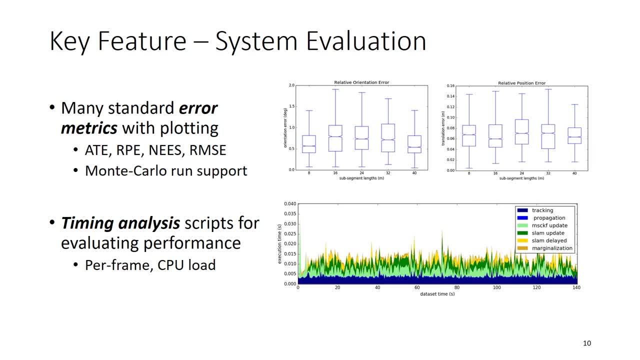 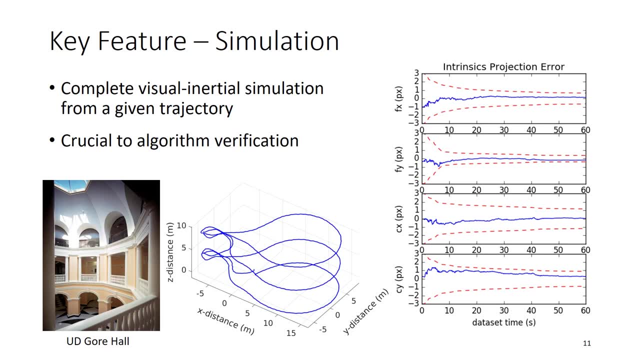 for evaluating performance on different devices, evaluating the per frame along with additional CPU load. We additionally have a complete visual inertial simulator and the input to this simulator is just a simple trajectory, And really this simulator is crucial for algorithm verification before you move to the real world and also ensuring that the estimator is estimating. 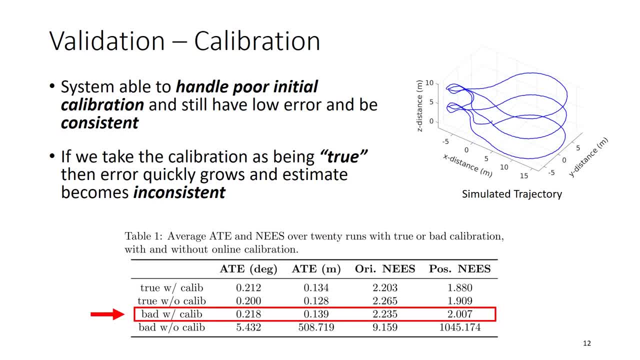 consistently. So, looking at some actual simulation results, we verified our ability to perform online calibration And what we found is that we're able to do a lot of work with the initial calibration. We're able to handle very poor initial calibration and still have low error. 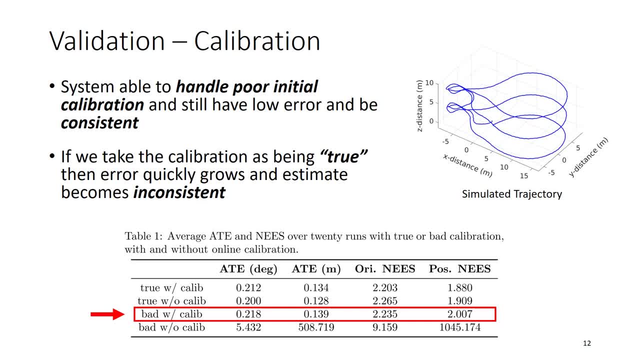 while being consistent. And so if you take a look at this table in the third row, we're able to start with very bad calibration and achieve the same level of ATE error as if we started with the true calibration. And the important part there is that we're not inconsistent. If we didn't perform this, 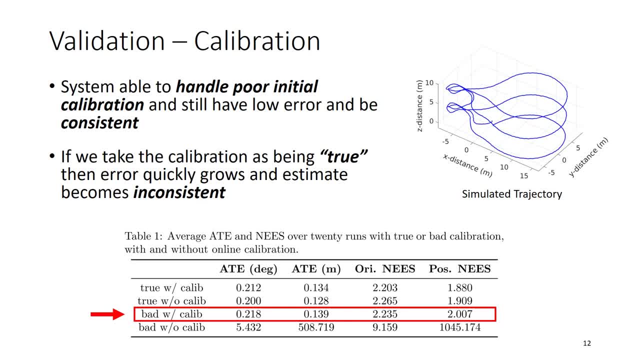 online calibration, our error would be very large and our estimator would become very overconfident. Looking at some other data, we're able to do a lot of work with the initial calibration and still have low error while being consistent, And so, if you take a look at this table, in the third row, we're able to. 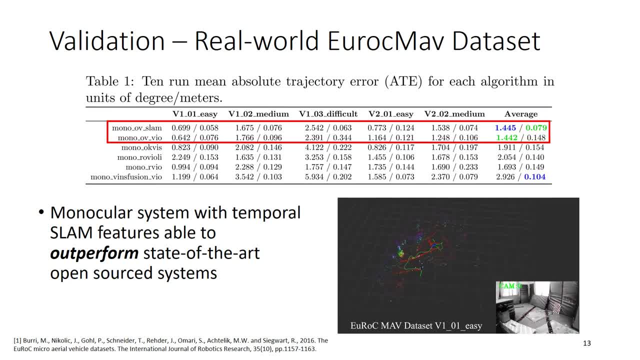 some real-world results. versus existing open-source systems, We are able to outperform state-of-the-art open-source systems. In this case we're on the URAC MAP dataset. Looking at another error metric, the relative pose error, we also show improvement over the. 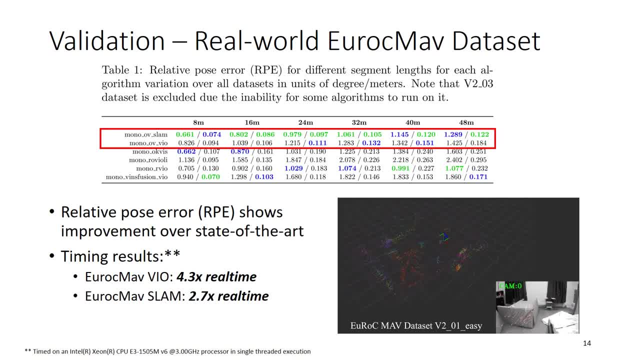 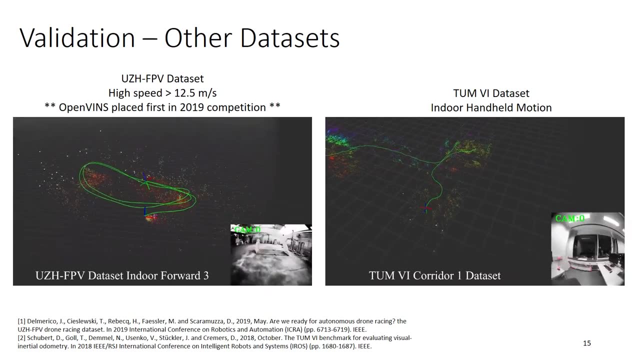 state-of-the-art, And one of the things I do want to draw attention to is that we are able to process faster than real time, single-threaded on a laptop CPU. We are able to run on a multiple other data sets. We are able to run on the UZHFPV data set, which is a very 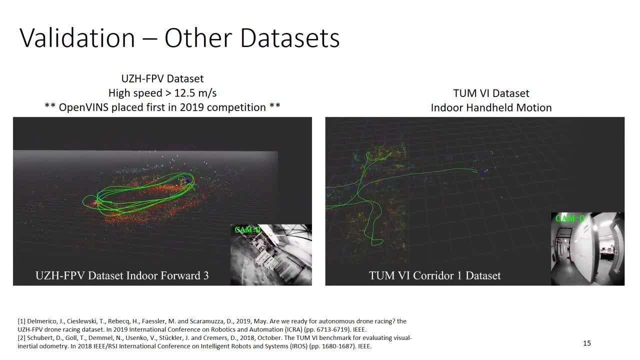 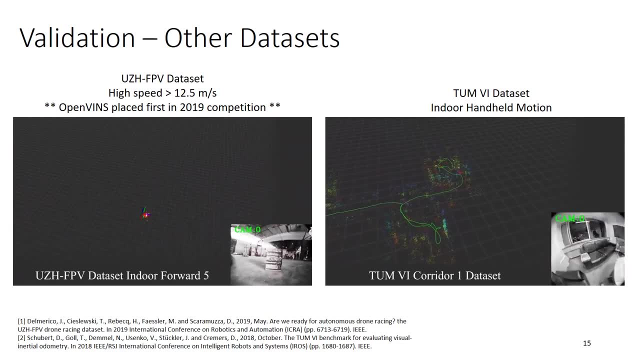 high-speed UAV data set. We did place first in the 2019 competition. Along with that, we are able to run on the TUMVI data set And these are really there along the URAC MAP. Any researcher that wants to come in can start running on on these data sets. 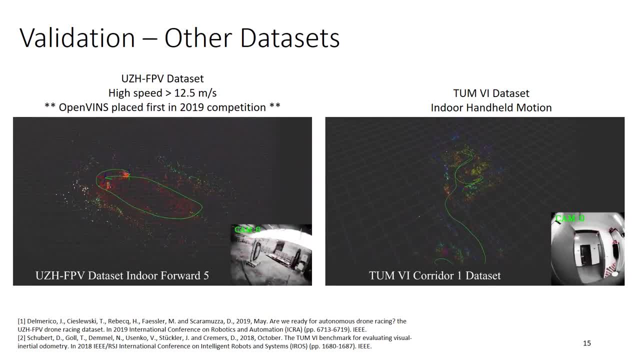 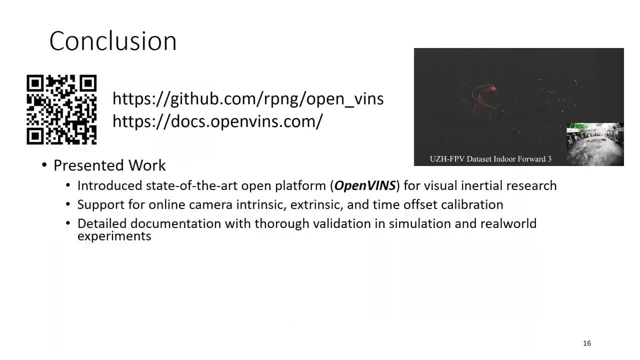 and can start evaluating and testing whatever improvements to visual-inertial state estimation that they can on any of these data sets. So, in conclusion, we've introduced a Salyard Open Framework, termed OpenVINZ, for Visual Notional Research. We support online camera, intrinsic, extrinsic. 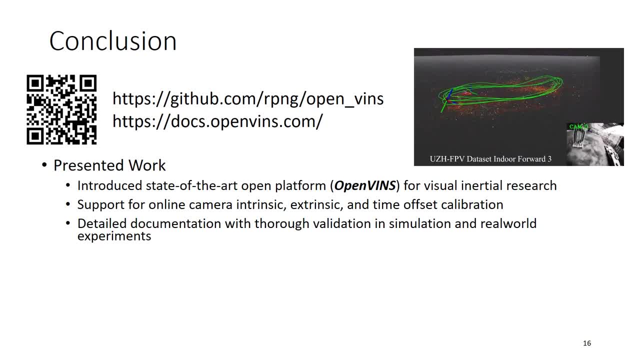 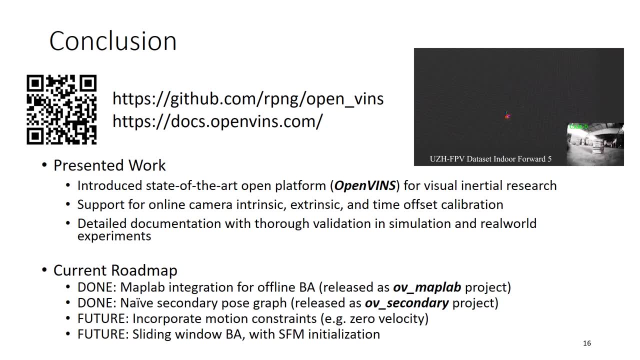 and time offset calibration. We have a very detailed documentation website and thorough validation and simulation and rewrote experiments. Looking into the future, there's a few items that we have already completed. We do have MapLab integration If you do want to run an offline VA after running OpenVINZ. 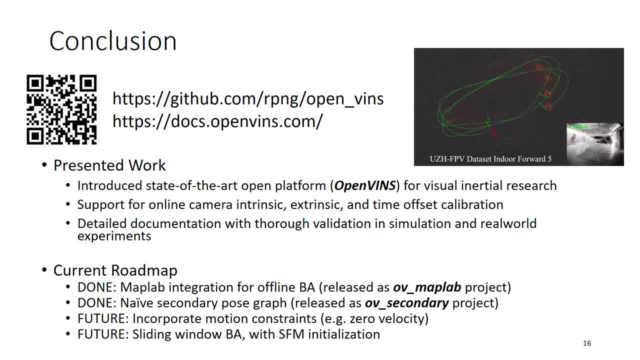 we have a very naive secondary pose graph released at the OV secondary project And in the future we want to incorporate motion constraints such as zero velocity updates, And we also want to include a sliding window, BA and structure for motion initialization into the repository. Thank you. 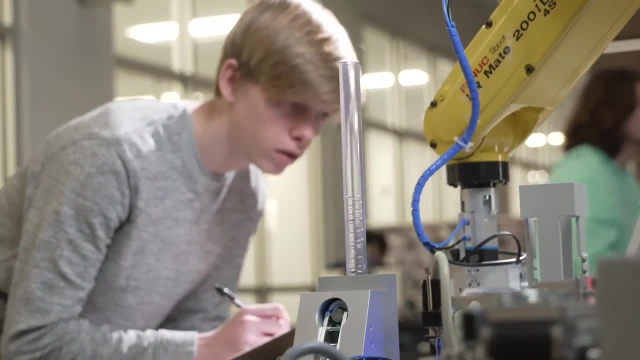 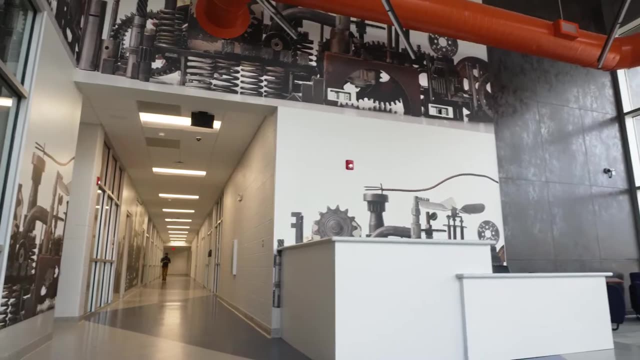 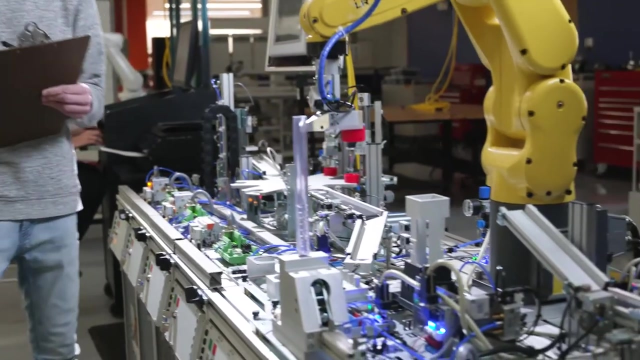 If you like working with your hands and if you like the challenge of doing something different each day, then I think you'll love mechatronics. We're here in the new facility located in T building in our advanced manufacturing center. Mechatronics is a word that replaces the old electro mechanical technician, The mech stands. 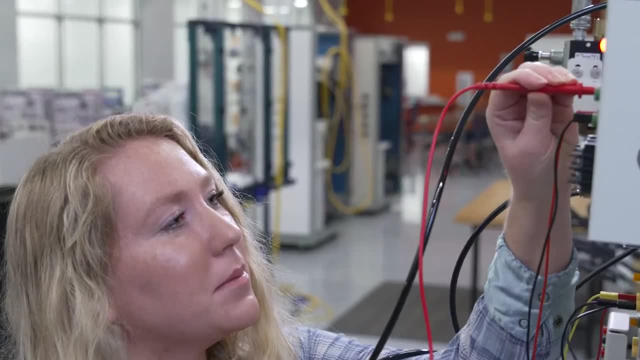 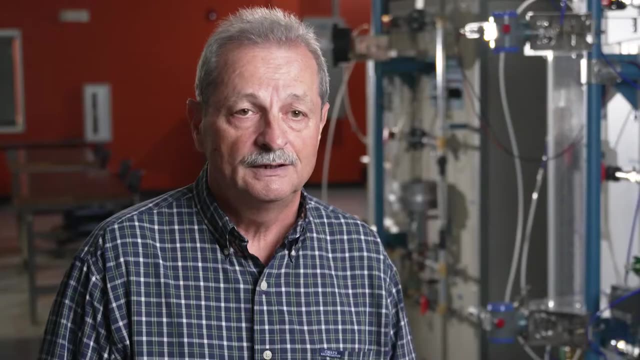 for mechanical and the tronics is representing the electronics or the electrical industry, Both of those working together. they're looking for folks that can do more than one thing. It's not just in the electrical field or the mechanical field. The reason I chose mechatronics was because the field that my dad is in